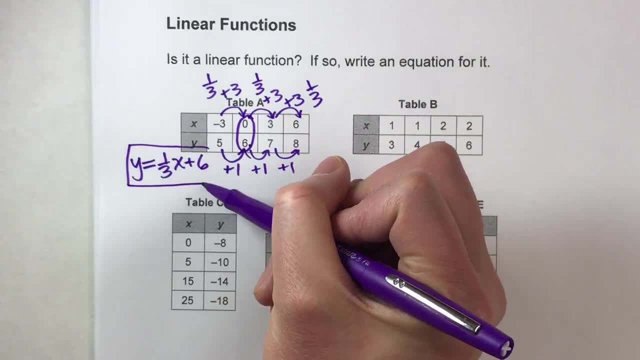 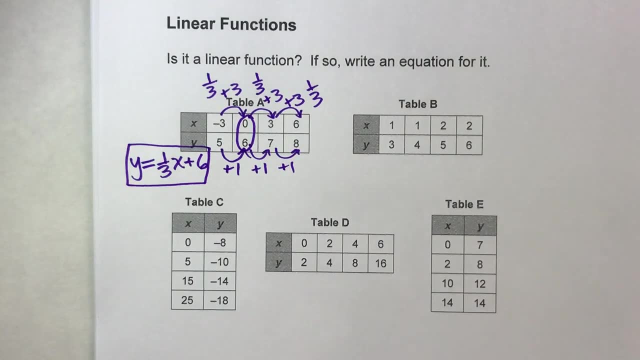 6 is my y value, so that's my y-intercept. There's the equation for this linear function: y equals 1 third x plus 6.. All right, And that's all we're going to do for each of these tables. Let's do table b to check it out. 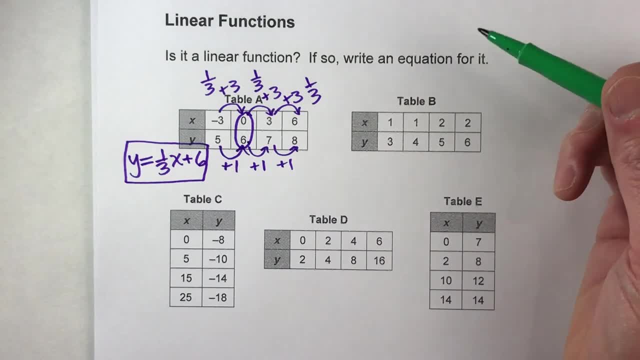 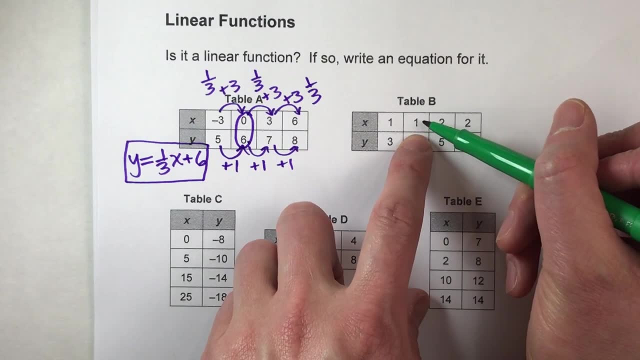 All right, so first let's check to see if it's a function For x, we've got 1.. Input of 1 gives us a 3.. Input of 1, again gives us a 4.. Uh-oh, Input of 2 gave. 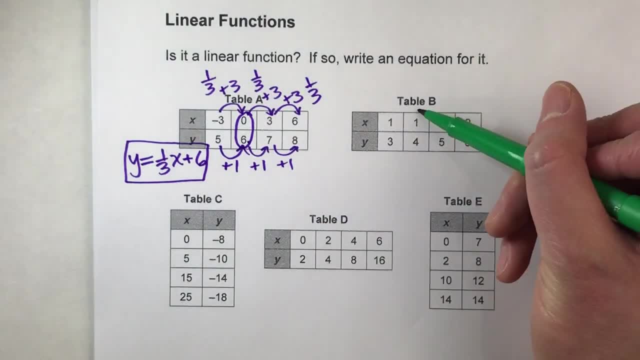 us a 5.. Input of 2 gave us a 6.. So notice, we've got an input of 1 giving us two different outputs, and an input of 2 gave us two different outputs. This is not a function. so, no, this is not a linear function. 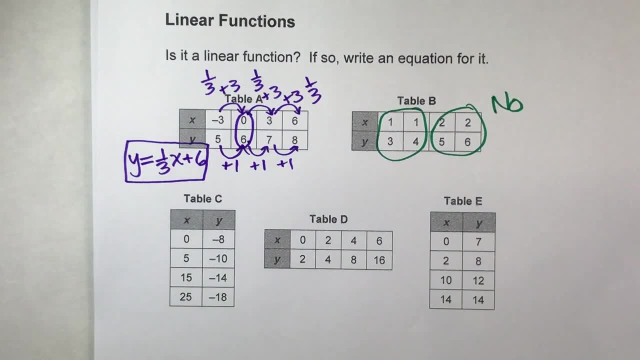 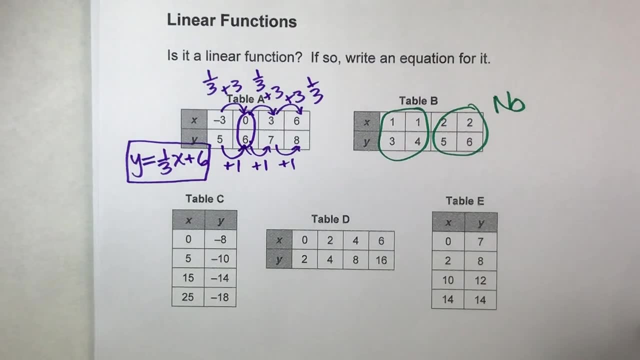 If it's not a function, it's definitely not a linear function, because the same input gave us two different outputs. All right, let's do another one. table C: Let's check to see if it's a function. Input of 0 gave us a negative 8.. 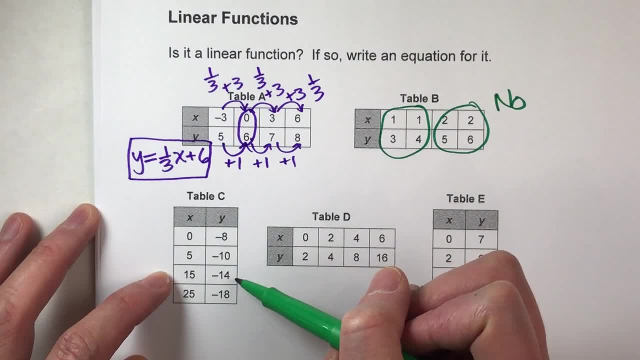 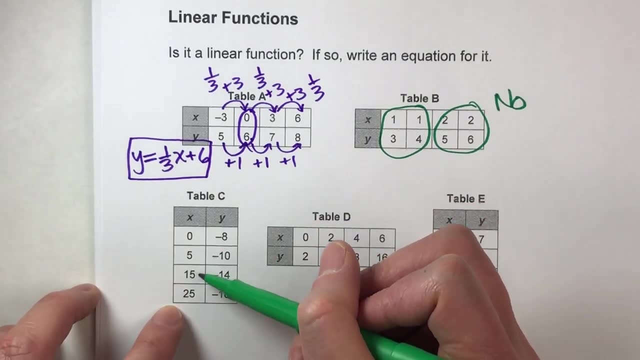 Input of 5 gave us a negative 10.. Input of 15 gave us negative 14.. And input of 25 gave us negative 18.. So notice, it is a function, because every single one of these x values gives us only one y value. 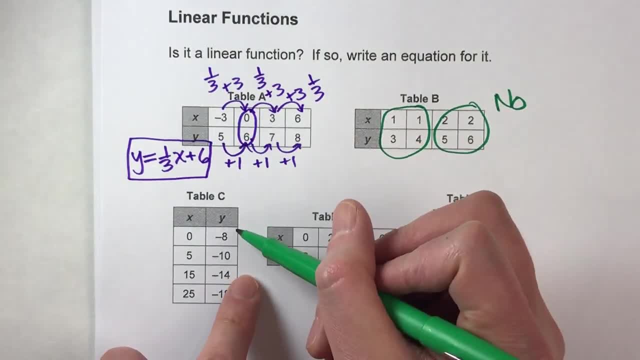 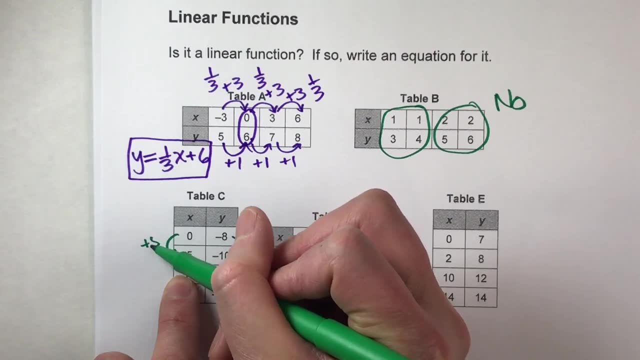 So now we can check to see if it's a linear. So let's find the rise. It goes down 2, and for these two my run is going from 0 to 5 and went up 5.. So my slope is negative 2. fifths: 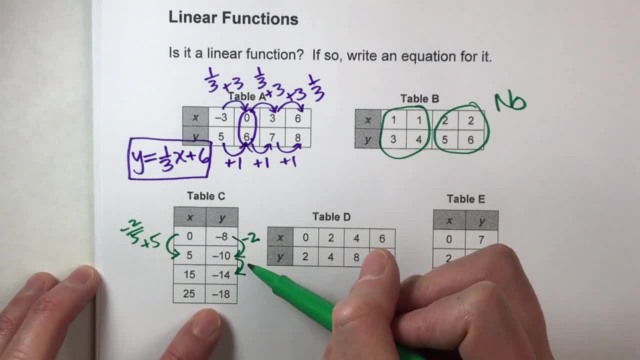 Okay, let's check the next two: From negative 10 to negative 14, it went down 4.. And my run goes from 5 to 15, so it went up 10.. So my slope is negative 4 over 10,. 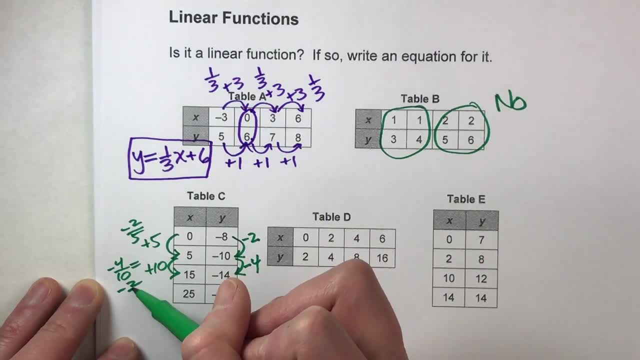 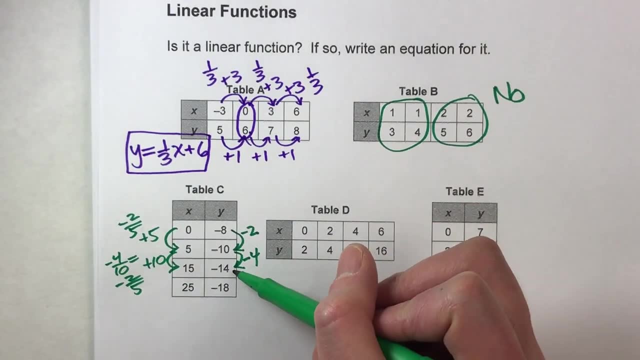 which reduces to negative 2 fifths. So so far it's consistent: negative 2 fifths, negative 2 fifths. Let's check the last one: Negative 4 to negative 18 went down 4.. From 15 to 25, it went up 10.. 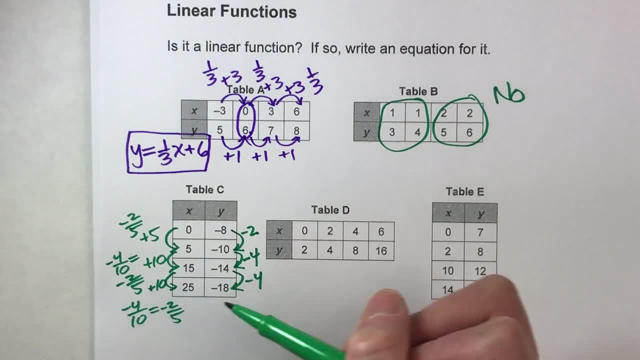 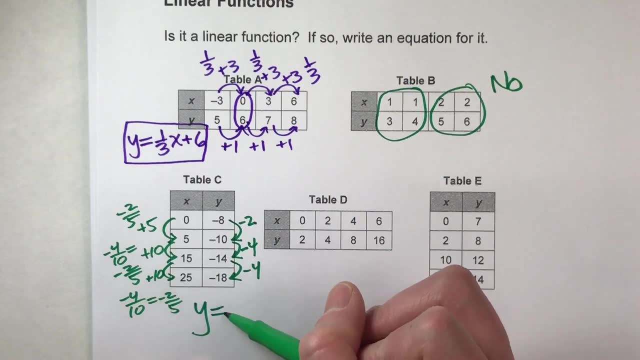 So negative 4 tenths again, which is negative 2 fifths. Hey, It's consistent. The slope is negative 2 fifths all the way throughout this table, So it is linear and we can write an equation for it now. 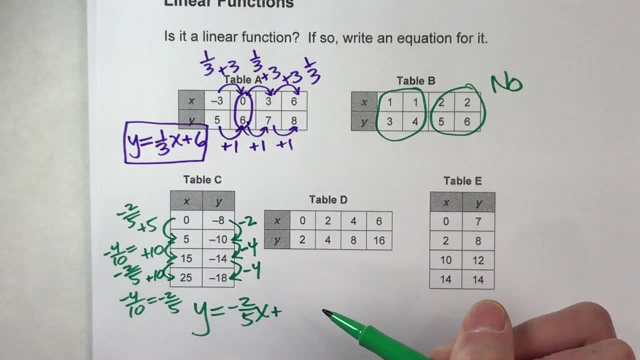 y equals negative 2 fifths x plus. now we need the y-intercept Find when x is 0.. y is negative 8, so plus negative 8.. There is our equation for that linear function. All right, Let's do table D. 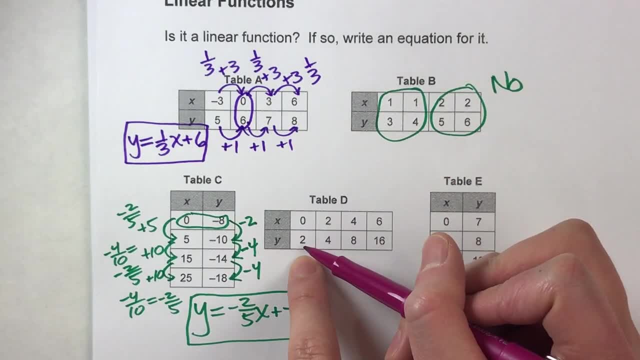 For table D. First, is it a function: 0 gives us 1, 2 gives us 1 output, 4 gives us 1 output and 6 gives us 1 output. Every single input gives us only 1 output. 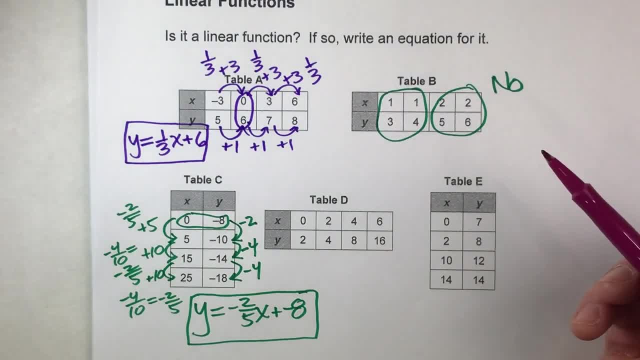 It is a function. Now let's check to see if it's linear. The rise goes up 2, and the run goes up 2.. So my slope is 2 over 2,, which is 1.. Now for this one, the rise is 4.. 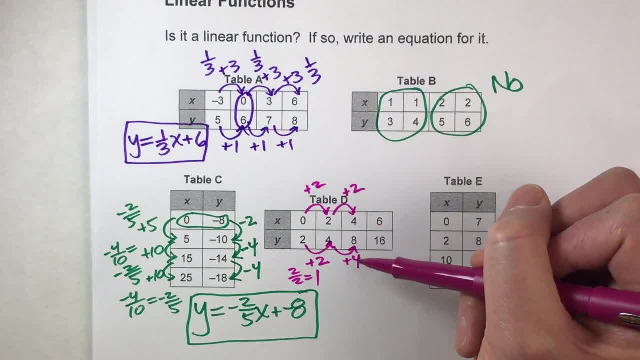 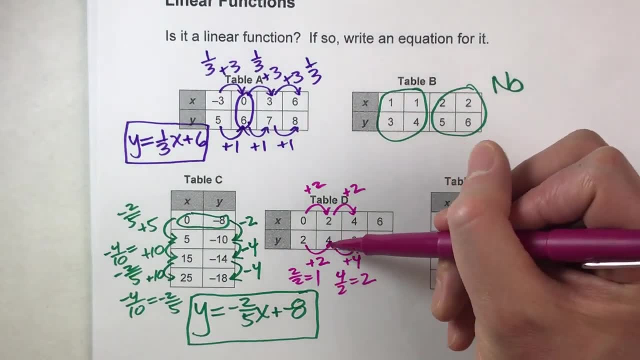 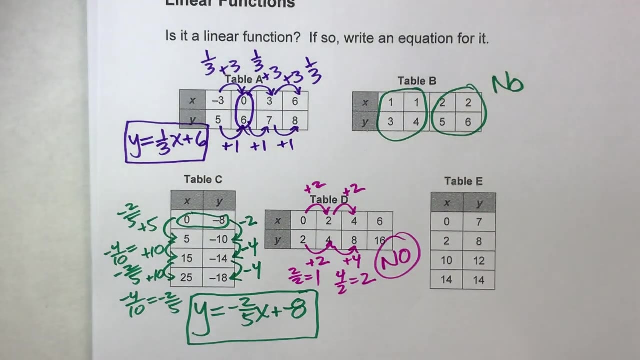 My run is 2,, so my slope is 4 over 2, which is 2.. Notice, my slope changed. It went from a slope of 1 to a slope of 2.. No, this is not linear, because the slope isn't consistent throughout the entire table. 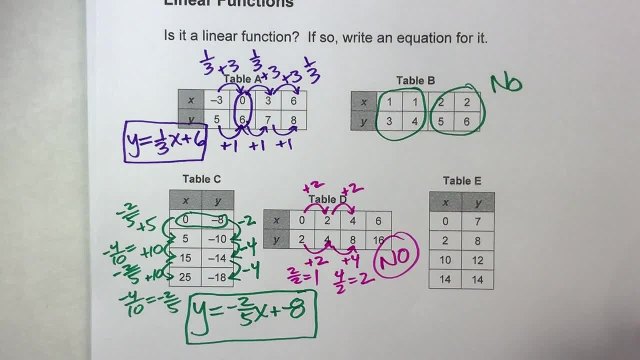 All right, We're on to the last one, then table E. So first off, is it a function? 0 gives us 1 output, 2 gives us 1 output, 10 gives us 1 output and 14 only gives us 1 output. 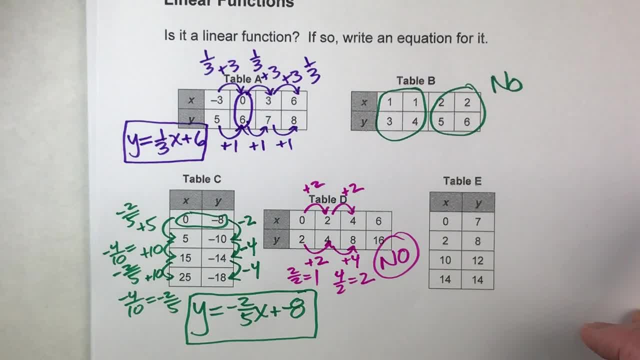 It is a function. Now let's check if it's linear. My rise is up 1,, my run goes up 2,, so my slope is 1 half, All right. next pair of rows, 8 to 12, went up 4, and my run went up from 2 to 10, up 8.. 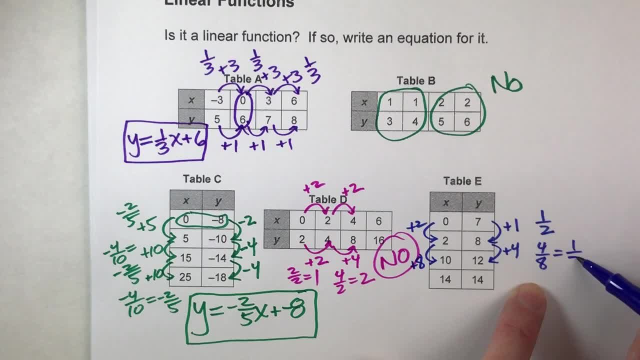 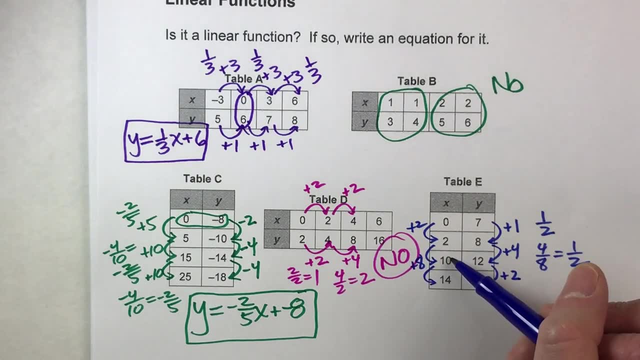 So my slope is 4 over 8. Which reduces to hey 1 half. It looks good so far. From 12 to 14, it went up 2.. My run went from 2 to 14, so it went up 4..